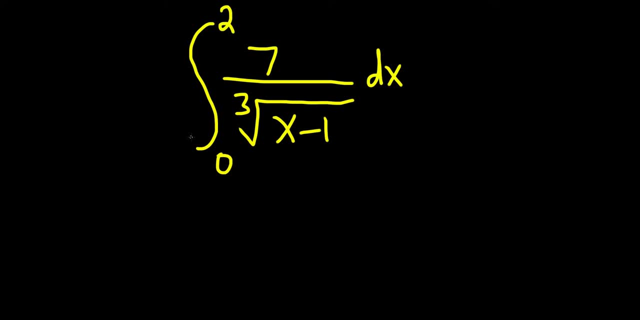 This problem. we have an integral and we're asked if it converges or diverges. and if it converges, you know, find the result. So this is an improper integral because it's not continuous at 1.. It has what's called an infinite discontinuity at 1.. If you plug in 1 here on the bottom of the 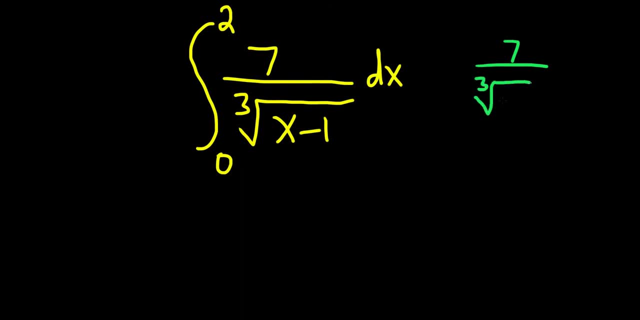 integrand you'll just get 7 over the cube root of 1 minus 1, which is 7, over the cube root of 0, which is just 7 over 0, which is undefined. So this function here is not continuous at 1 and. 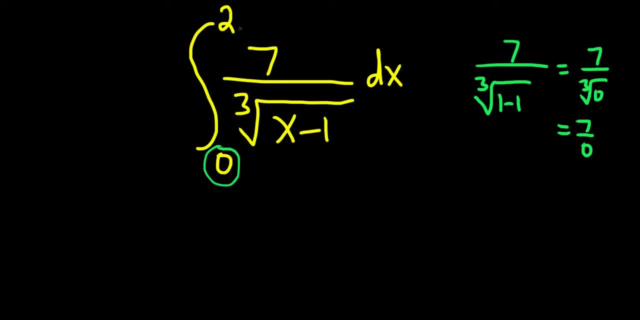 1 is between 0 and 2. right, Those are your limits of integrations. This is an improper integral. So, to do this problem, what we're going to do is we're going to break it up at 1, because 1 is the problem. area 1 is where you have the discontinuity, So let's write this as two. 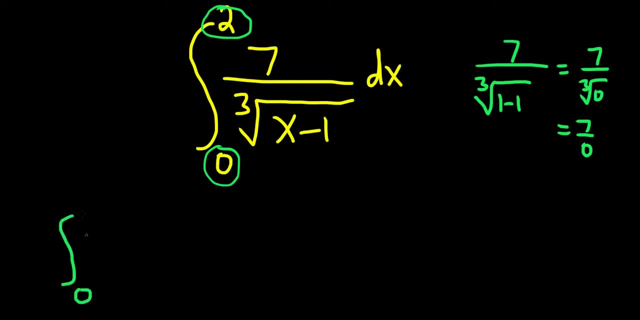 integrals. So we'll write it as the integral from 0 to 1.. 7 over the cube root of x minus 1 dx, plus the integral from 1 to 2.. So instead of just going straight from 0 to 2, first we go from 0 to 1 and then we go from 1 to 2.. This is 7 over the cube. 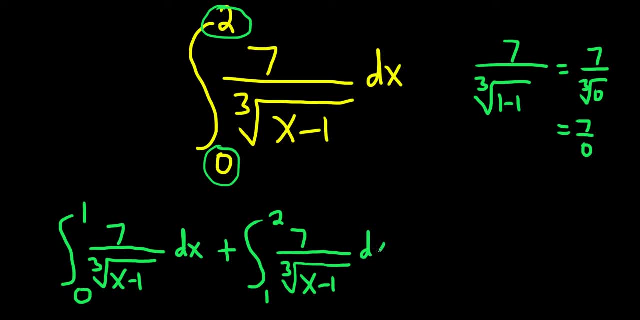 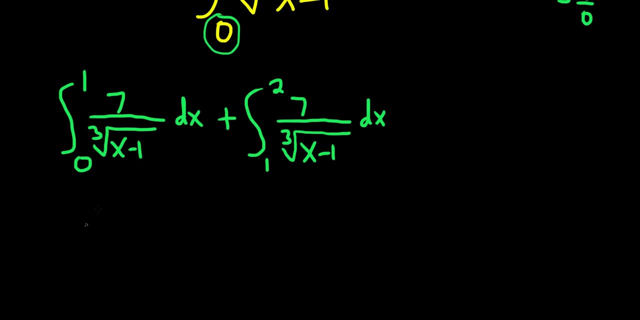 root of x minus 1 and again dx. All right, now, it's carefully, carefully do this. So the problem area is at 1.. So what you do is you basically replace the number where there's an issue with a variable. So I like to use the letter b, So I'm going to. 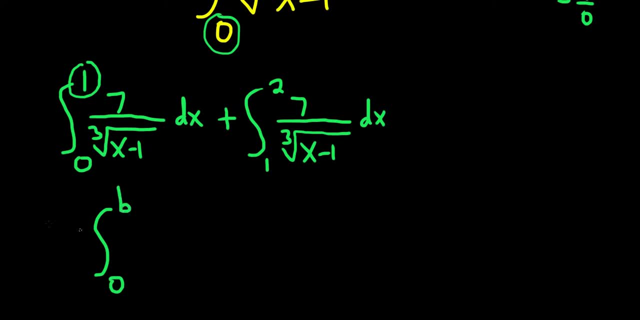 use a 0 here and put a b here, Okay, and then put a limit here, So you replace the 1, because 1 is the discontinuity, and then you approach 1 with your b. Now, to figure out which direction you approach from, you have to. well, you can think about it like this. You can think about it like: 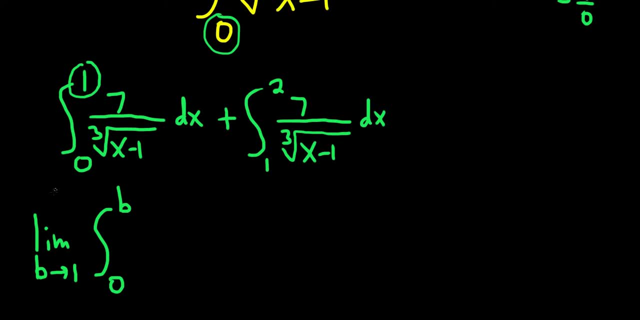 intuitively, or you can draw a picture and do it intuitively. Intuitively, you're approaching from the left, because you're going from 0 to 1 and you're approaching 1.. If you want to look at a picture, what you can do is you can plot the 0, you can plot the 1 and the b is always in the middle. 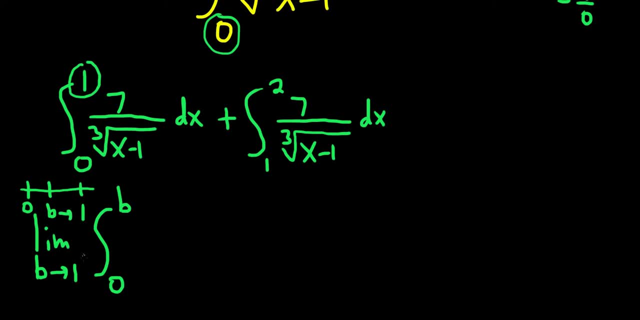 and so b is approaching 1.. Ah, okay, so it's approaching from the left. You see, from the picture will always tell you which way it's approaching from. I'm going to go ahead and make a lead here. So I'm going to go ahead and make a lead here. So I'm going to go ahead and. 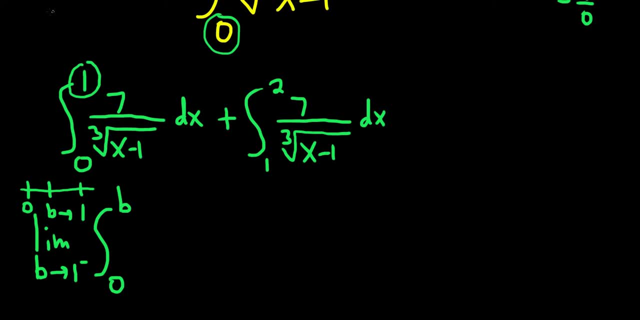 make a lead here. I'm going to rewrite this in a way that allows us to integrate it. So first, notice that a cube root can be written as a 1, 3rd power. So we can write the integrand like this: and then, if you bring it up, what happens is the exponent becomes negative. So I'm going to write: 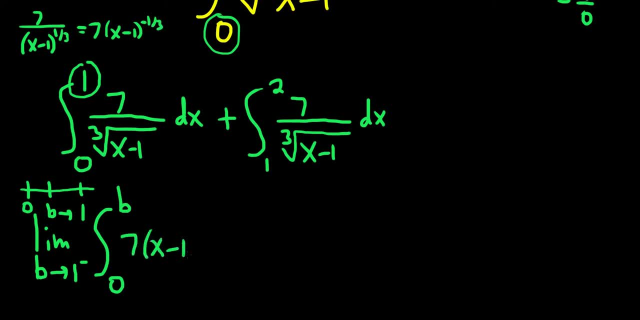 this like that. So 7 x minus 1 to the negative 1. 3rd: This is for the next step, so when we have to integrate it, we don't have to do a bunch of extra steps. Same thing here: we replace the 1 with a letter and you can use the same letter. it's okay, I'll use b. 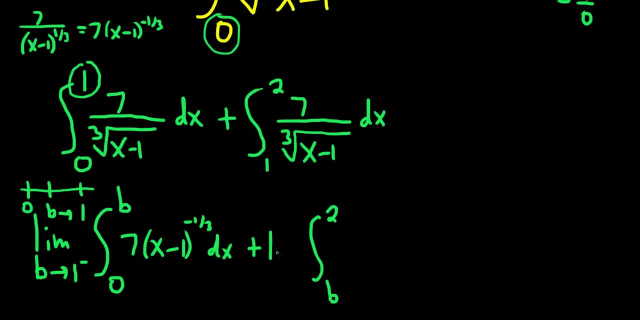 here and there's a 2 here, and this is the limit. as b approaches, 1 again, Except this time it's a little bit different, Let's see. so here's 0. oh no, here's 1 and here's 2. right, we're using these. 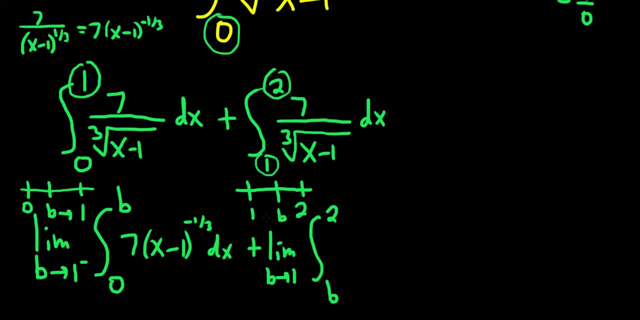 limits now, and so b is here. So you see that b is approaching from the right this time. so it's a plus symbol, and this is 7. x minus 1.. This is one of the harder ones. if you're, if you're doing this for a class, if you're studying. 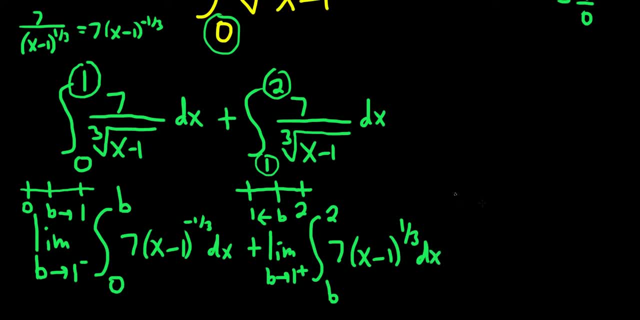 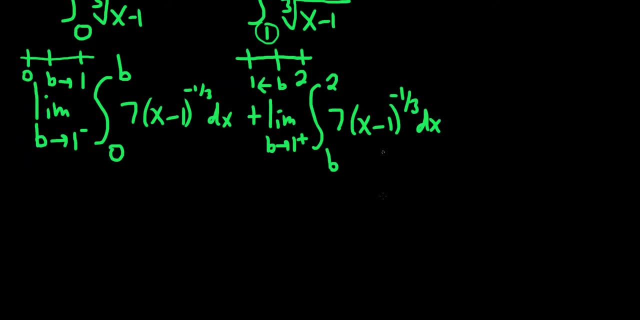 some calculus. I would consider this one of the harder problems that you typically see in a calc 2 class. That's a little mistake. there is a minus. Alright, so to integrate this, we're technically supposed to make a u substitution. You would let u equal x minus 1 and then so du is just dx. So 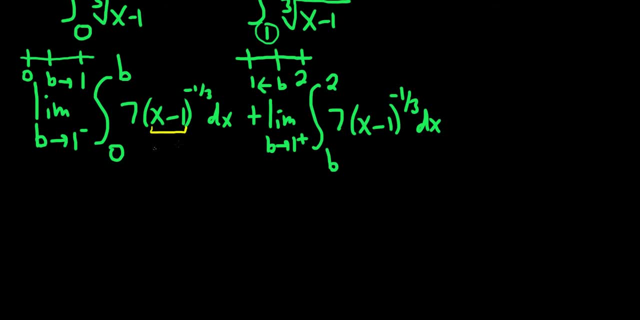 because du is just dx, nothing else is going to happen. so we can be a bit abusive here and just integrate it without making a? u sub. So this is the limit. so we still have that limit. as b approaches, 1 from the left of 7, and then we have x minus 1. we're adding 1, so negative 1. 3rd plus 1. 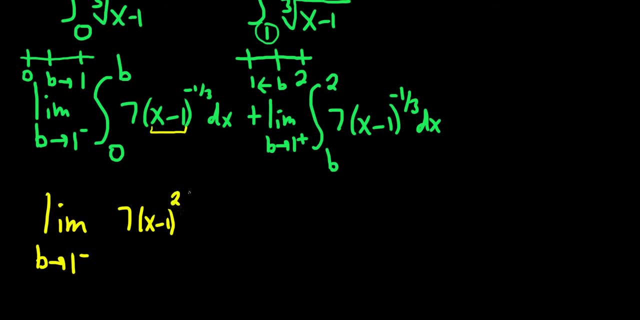 is negative: 1 3rd plus 3- 3rds, which is 2- 3rds. and when you divide by 2- 3rds, you really multiply by 3 over 2.. That's the power rule. We're dividing by 2- 3rds so that results in a. 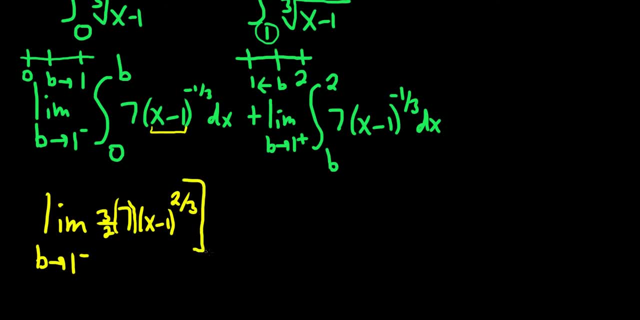 multiplication by 3 halves and we're going from 0 to be heavy on the notation. plus limit b approaches 1 from the right. Same thing. let's integrate this bad boy. this is 7 x minus 1. the integration is exactly the same, so it's negative. 1 3rd plus 3 3rds, which is 2: 3rds. 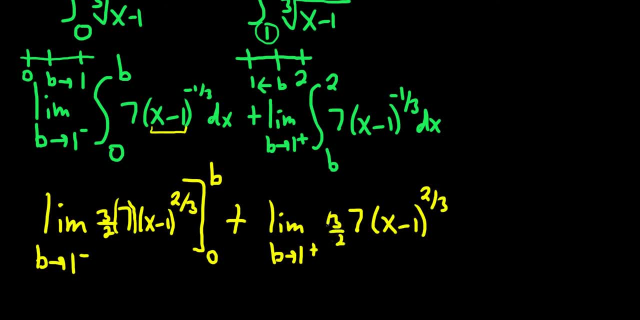 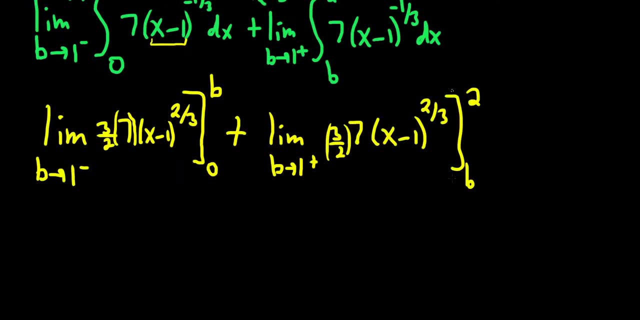 We divide by 2 3rds, so we really multiply by 3 halves, except this time we're going from b to 2.. Okay, let's keep going. It's a pretty wicked problem. So this is the limit. Okay, this is the. 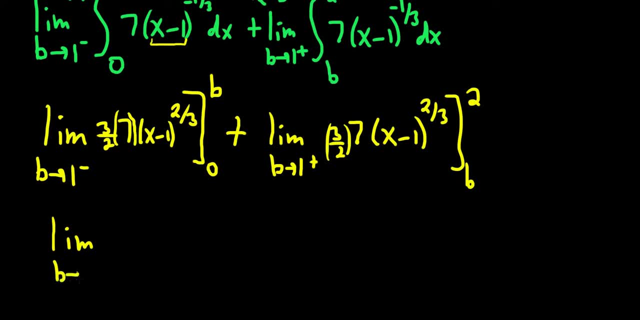 limit as b approaches 1 from the left. So let's see, this is going to be 3 times 7 is 21, so this is 21 over 2.. Okay, so I'm going to leave it like this: 21 over 2.. Whoops, 21 over 2, and let me just 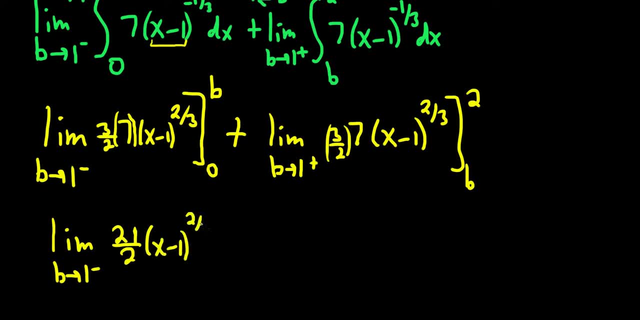 show an extra step here. I'm just going to. All I did here was multiply the 3 halves times the 7. I'm just taking a breather here and just slowing down, So I'm rewriting everything and just doing the multiplication here, So approaching 1. 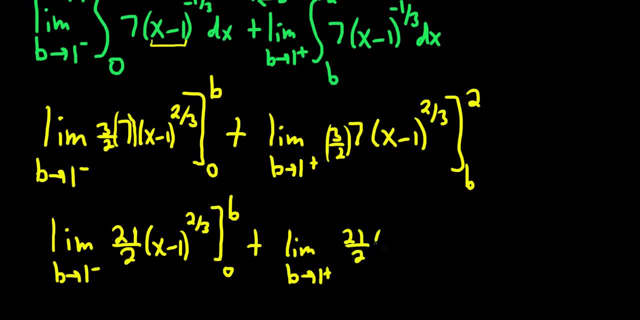 this is 21 over 2.. I thought this problem was going to be a little bit harder, but I think it's going to work out. I think this is going to converge. Originally I was thinking, oh, this is one of the divergent ones. but no, no, this is this. 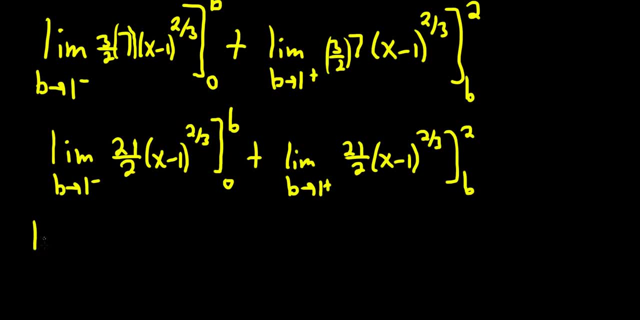 this thing is going to converge, so it's not so bad. So this is the limit as b approaches, 1 from the right. All right, so first you plug in the b, so I'll leave the 21 halves here, So we'll get b minus 1. 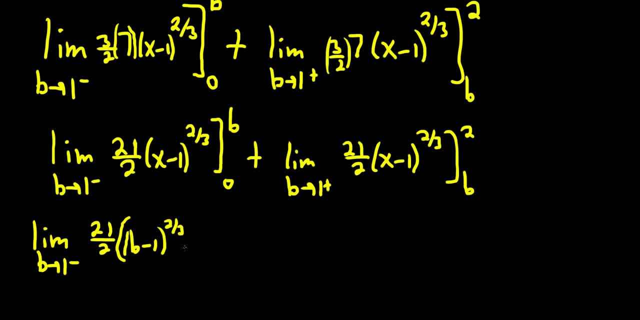 to the two-thirds minus and then you plug in 0.. So 0 minus 1 to the two-thirds, Okay, just like that, Boom, Okay. so plug in b for the x subtract, plug in 0 for the x Boom, and then left the 21 halves. 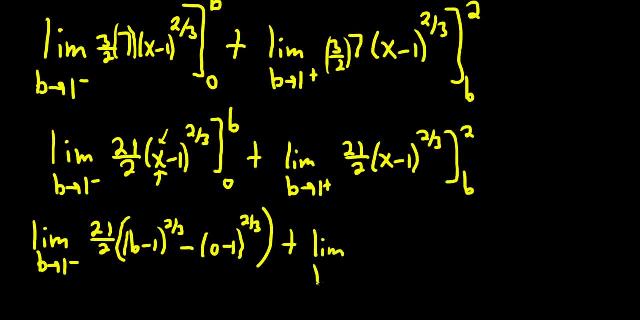 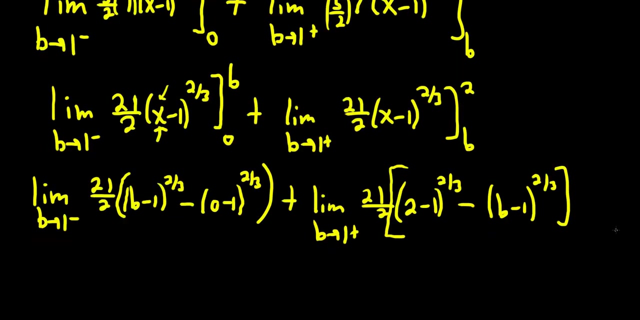 out. plus we have another limit here: b approaches 1 from the right, So 21 halves. this will be 2 minus 1 to the two-thirds minus. I'll put a bracket here- minus, and then b minus 1 to the two-thirds. Ridiculous on the notation. All right, it's. 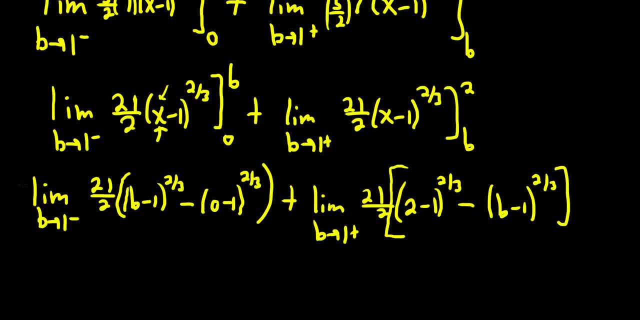 crazy. So let's see what happens here. So I think now we can take the limit. So actually we can just plug in 1, which is really nice. So I think that's it. Oh, and then we can plug in b 25 to the x, to the y. 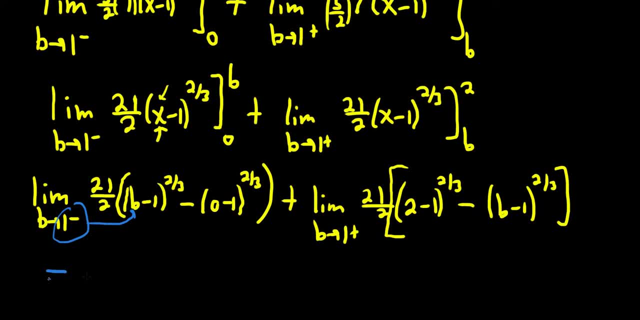 So if you plug in b, 25 to the x, 25 to the y to the y, I think now we can take the limit. So actually we can just plug in 1, which is really nice. If you just plug in 1 here, you drop the limit sign now. so this is equal to 21 halves, okay. 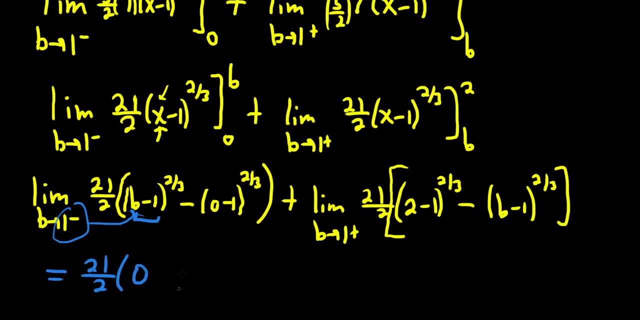 1 minus 1 is 0 when you plug in a 1 here, so this is just 0, and then minus negative 1 to the 2 thirds plus, and then 21 halves. 2 minus 1 is 1, so 1 to the 2 thirds is 1,. 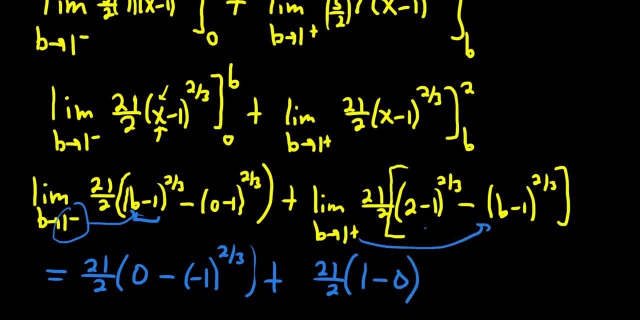 and then plugging in 1 here, it's 0 again, boom. So again, 2 minus 1 is 1, so you get 1 to the 2 thirds, which is just 1, and then plugging in 1 here would give us 0.. 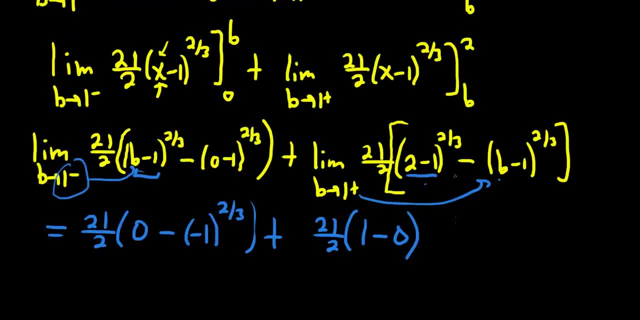 All right. So let's see what happens here. This is equal to so negative 1 to the 2 thirds. we should investigate what that is. So if you have negative 1 to the 2 thirds, what you do is you take the cube root of negative. 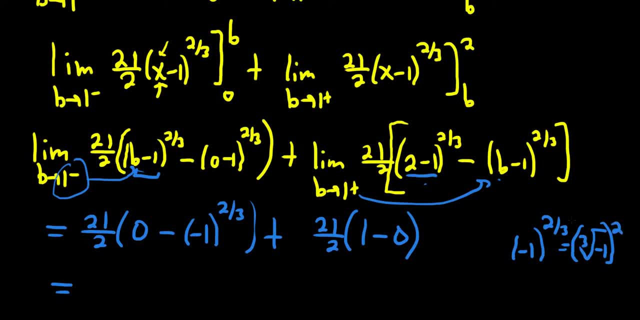 1. one and you square it. that's how it works. this number here goes in the little pocket, always cumulative. negative one is negative one. okay, so this is negative one squared. so you just get one. so this is just one, but there's a negative, so this will be. this is a positive one, but there's a negative here. 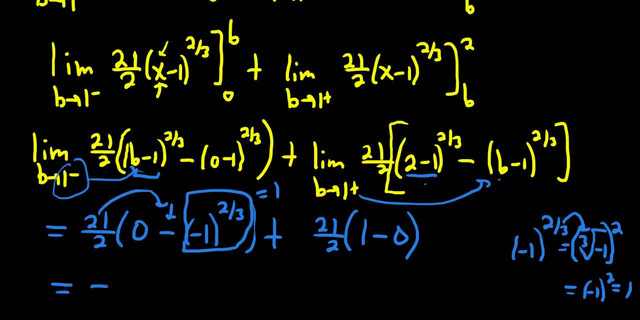 then there's a 21 halves, so that'll be negative 21 halves, and then this one over here is plus 21 halves. oh, look at that, so you get zero. boom, that is certainly a number, so this thing converges awesome problem. so, yeah, really really good stuff. I hope this video has been helpful.